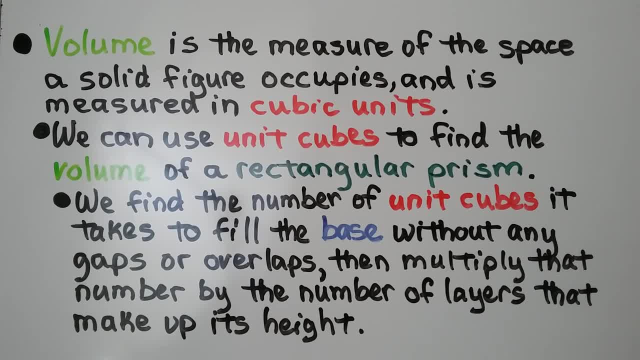 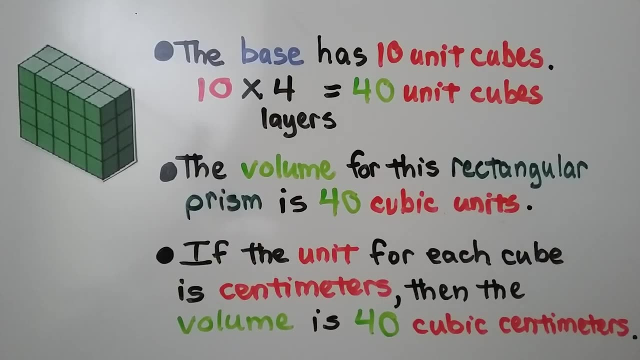 We can use unit cubes to find the volume of a rectangular prism. We find the number of unit cubes it takes to fill the base without any gaps or overlaps, then multiply that number by the number of layers that make up its height. Here's a rectangular prism and the base has 10 unit cubes. 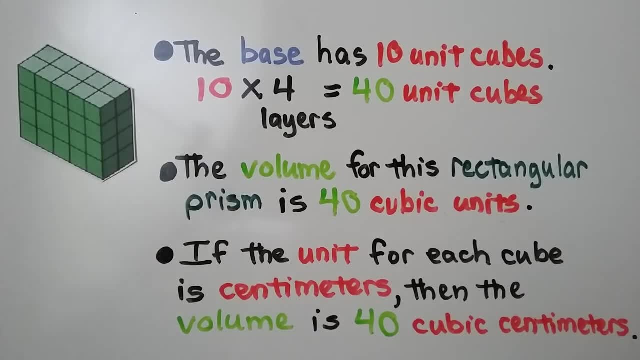 There's four layers. We do 10 times the four layers, That's equal to 40 unit cubes. So the volume for this rectangular prism is 40 cubic inches. If the unit for each cube is centimeters, then the volume is 40 cubic centimeters. 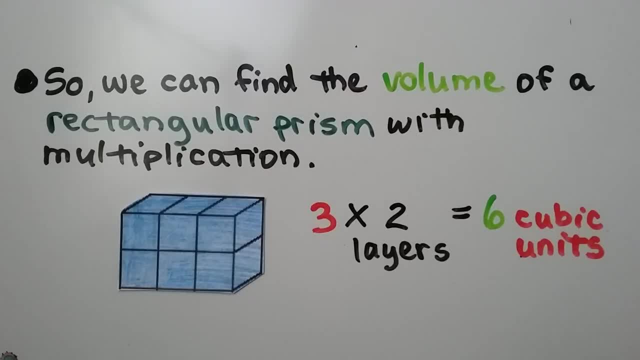 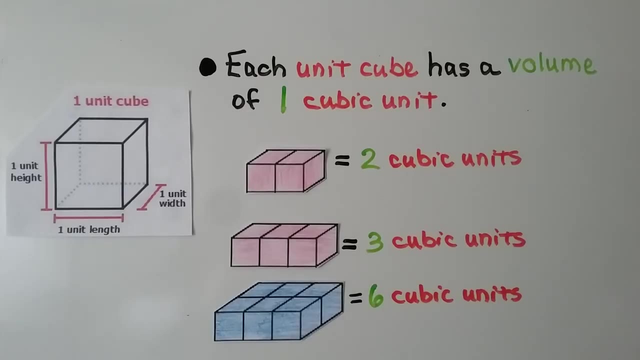 So we can find the volume of a rectangular prism. with multiplication We have three unit cubes. There's two layers. Three times two is equal to six cubic units. Each unit cube has a volume of one cubic unit. It's one unit length, one unit width, one unit height. 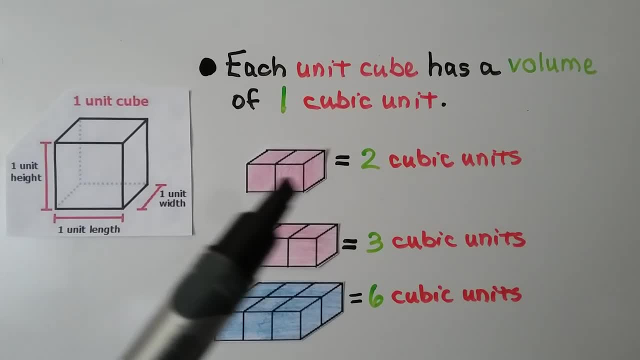 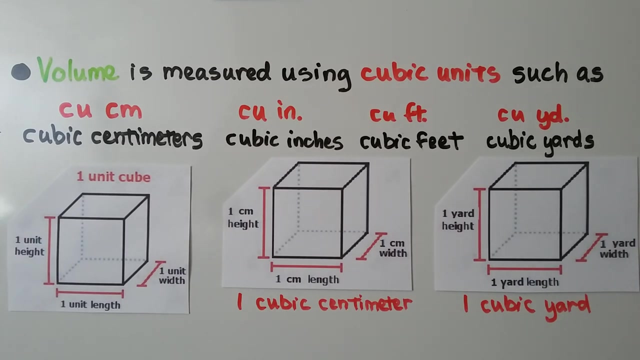 It's a one unit cube. If we have two of them, it's two cubic units. If we have three of them, it's three cubic units. If we have six of them, it's six cubic units. Volume is measured using cubic units such as cubic centimeters, which is abbreviated as a Cu. 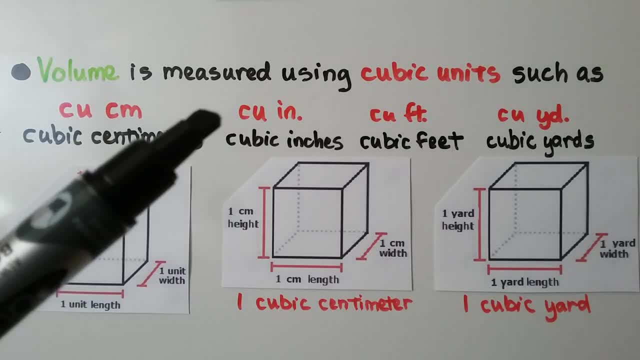 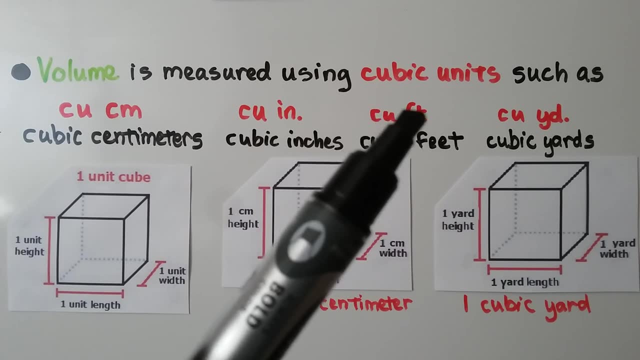 for the cubic and Cm for centimeters, Cubic inches, Cu for cubic, In period for inches, Cu for cubic, Ft for feet, Ft period. And we have cubic yards, That's Cu for cubic and Yd period for yards. 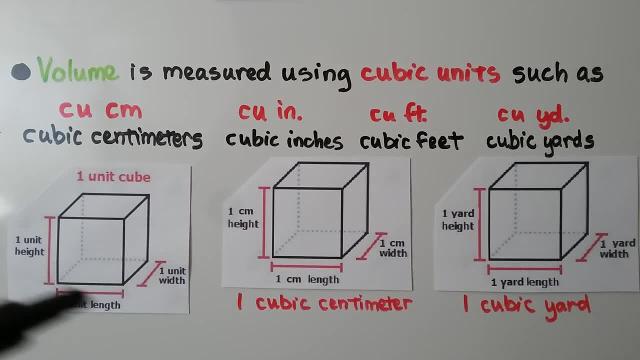 So a unit cube is a unit length, unit width and a unit height. If they were centimeter units, it would be one centimeter length, one centimeter width, one centimeter height. That would be one cubic centimeter. If the units were yards, it would be one yard in length, one yard in width and one yard in height. 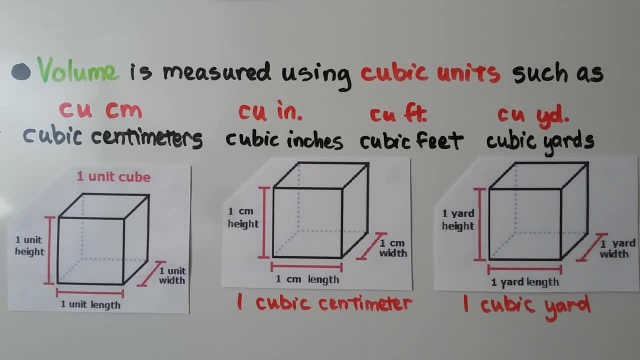 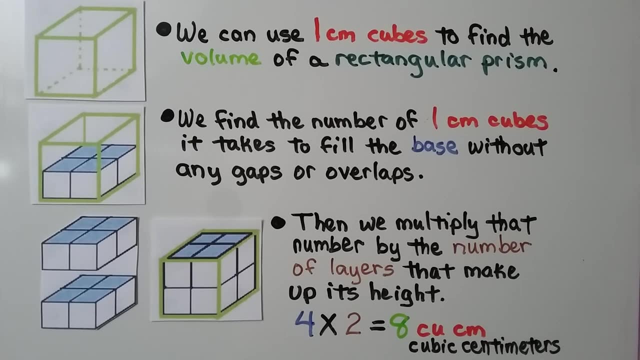 And it would be one cubic yard. We can use one centimeter cubes to find the volume of a rectangular prism. We find the number of one centimeter cubes it takes to fill the base without any gaps or overlaps. Then we multiply that number by the number of layers. 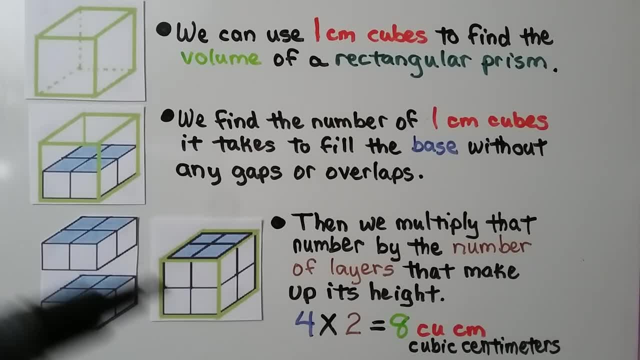 that make up its height. There's two layers. We have four on the first layer. That's 4 times 2 layers. That's equal to 8 cubic centimeters. So it's cubic centimeters, because we said they were 1 centimeter cubes. 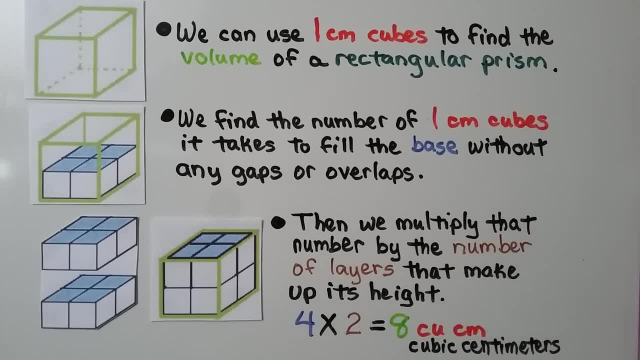 The volume of this rectangular prism is 8 cubic centimeters. The volume of this rectangular prism is 8 cubic centimeters. When unit cubes are stacked, we may not see it. The volume of this rectangular prism is 8 cubic centimeters. 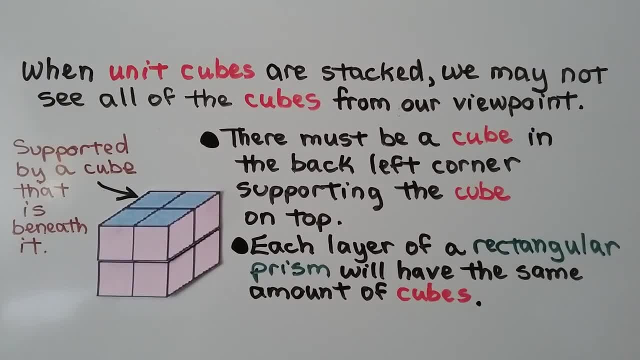 not see all of the cubes. from our viewpoint. We look at this one. There must be a cube in the back left corner supporting this cube. on top It's supported by a cube that's beneath it, And each layer of a rectangular prism will have the same amount of cubes. So if we lifted the layer away, we'd see that. 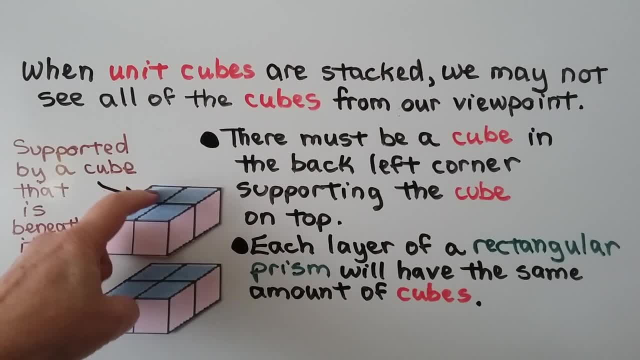 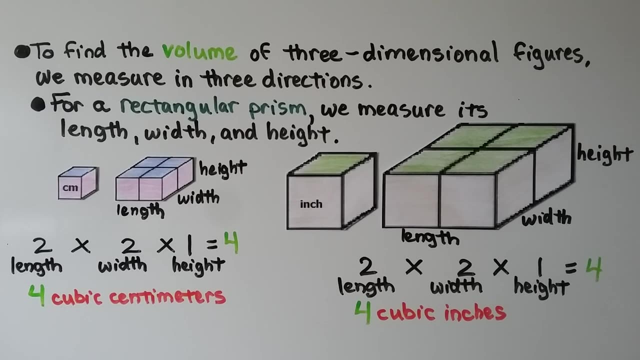 this was the one that was hiding. It was supporting this one above it. See To find the volume of three-dimensional figures. we measure in three directions. For a rectangular prism, we measure its length, width and height. So here we have. 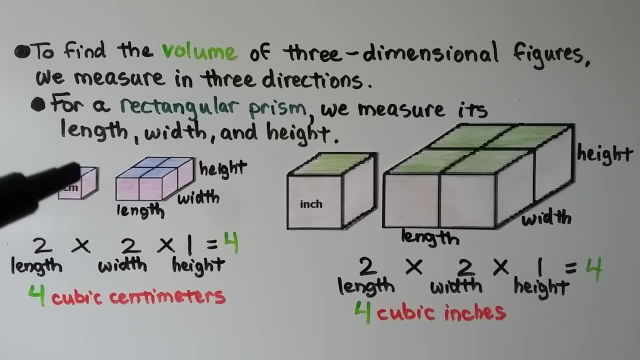 a one centimeter cube. Here there are four of them. We measure the length: There's two centimeters in length. The width is two, so that would be two centimeters, And the height is one, so that would be one centimeter. We multiply the length times the width, times the height, Two times two. 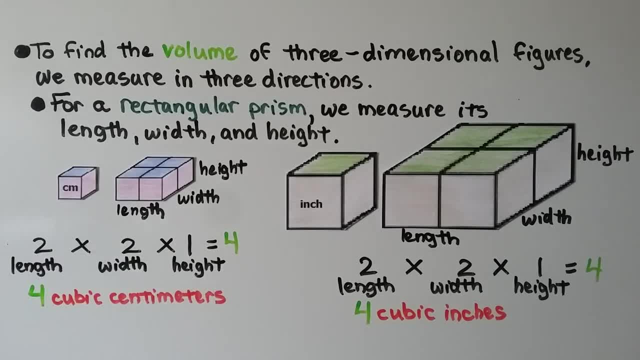 is four. Four times one is four, That's four cubic centimeters And we have a one inch cube. so the length is two inches, the width is two inches and the height is one inch inch. and we have the same multiplication 2 times. 2 times 1 is 4, except because these 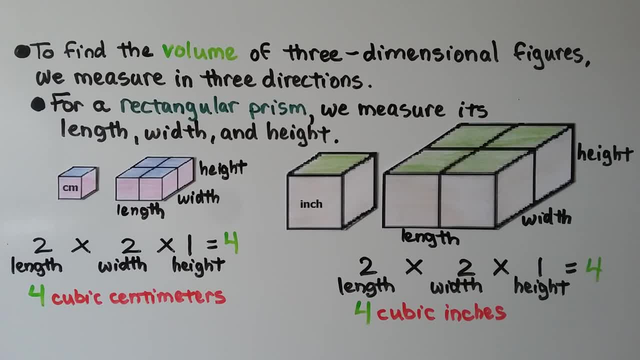 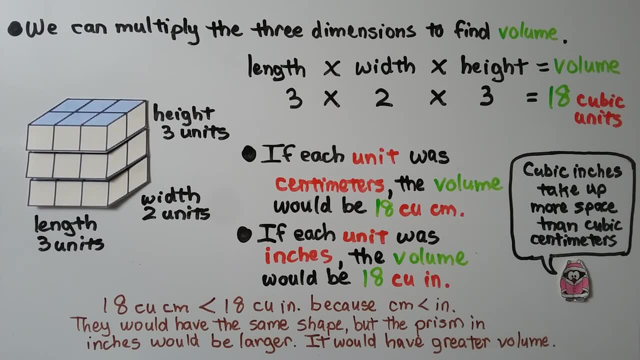 are inches, we have 4 cubic inches. We can multiply the three dimensions to find volume. Length times width times height equals volume. We have a length of 3 units, we have a width of 2 units and we have a height of 3 units. 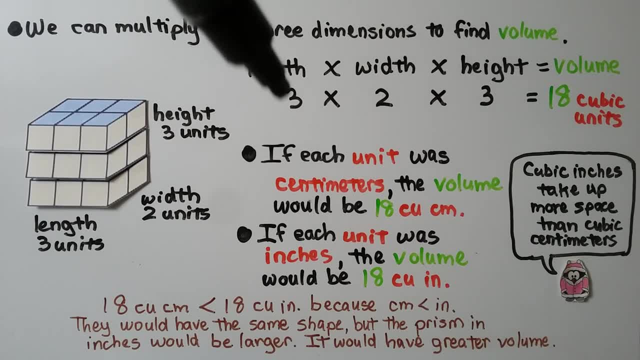 We do 3 times 2 times 3.. 3 times 2 is 6, and 6 times 3 is 18, that's 18 cubic units, And if each unit was centimeters, the volume would be 8 cubic centimeters. 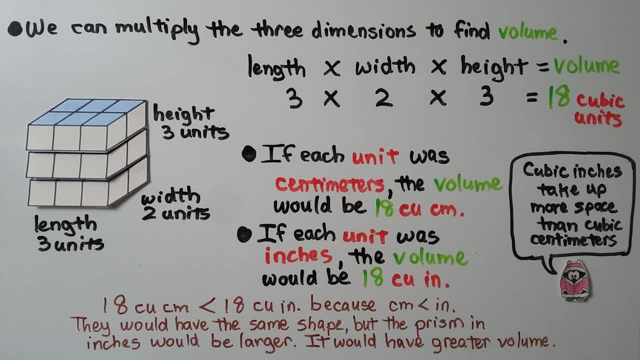 And if the unit was inches, the volume would be 18 cubic inches. So we have three layers here. We can see them. If I move these up, Okay, You'll see the three layers. We have 6,, 3 times that's 18 cubic units. 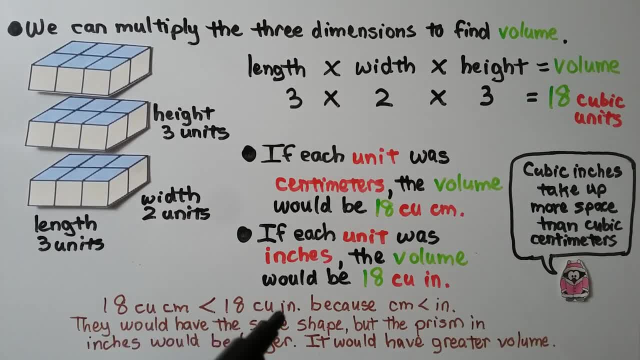 And 18 cubic centimeters is less than 18 cubic inches, because centimeters are less than inches. They would have the same shape, but the prism in inches would be larger. It would have greater volume. Inches are larger, So cubic inches take up more space than cubic centimeters. 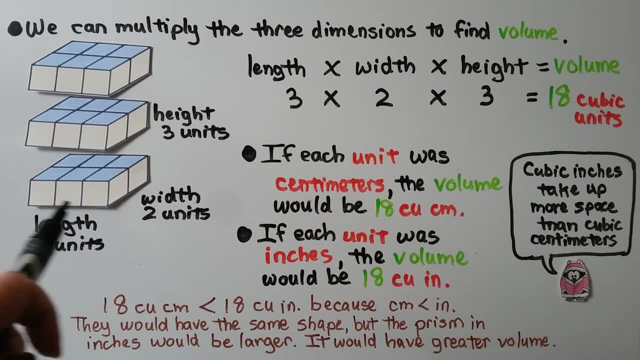 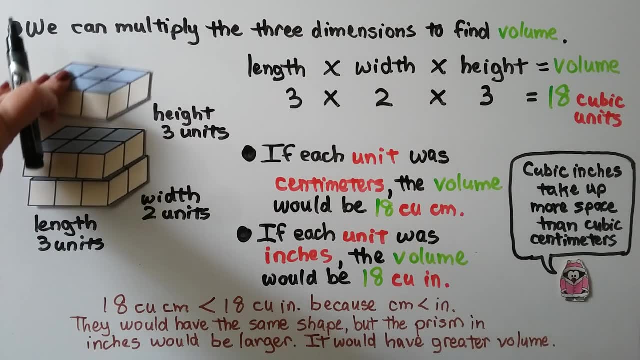 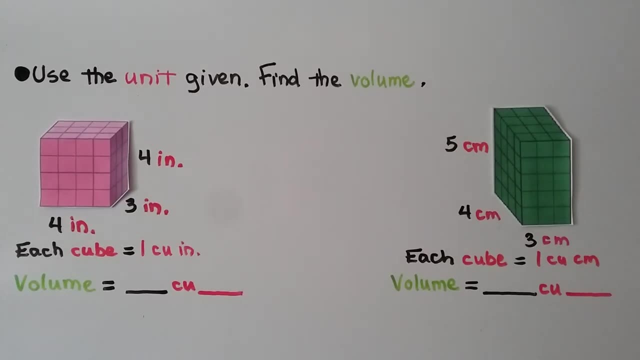 So we multiply the length of 3 times the width of 2 times the height of 3 units. We multiply the length of 3 times the width of 2 times the height of 3 units. Use the unit given, find the volume. 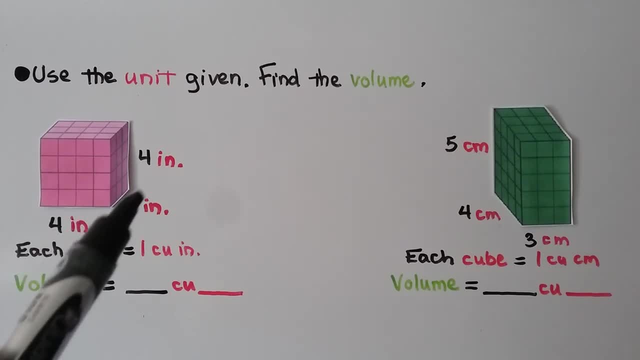 So this is in inches. It's saying that this is 4 inches, this is 3 inches and this is 4 inches because it's got 4 layers. So each cube is 1 cubic inch. We can multiply 4 times 3.. 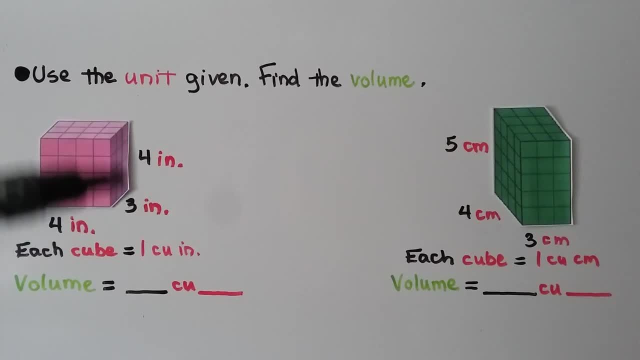 That's 12.. And we multiply it by the layers, There's 4 layers. 12 times 4 is 48.. Each cube is 1 cubic inch. It's 48 cubic inches. This one is in centimeters. Each cube is 1 cubic centimeter. 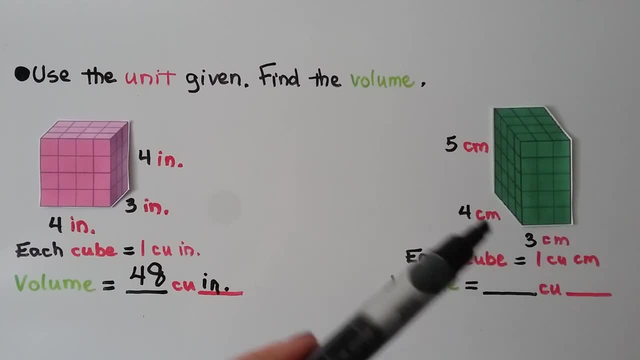 We have 3 centimeters this way For length. we have 4 centimeters For width. we have 5 centimeters For our height. we can do 3 times 4.. That's 12. Times the height, 5.. 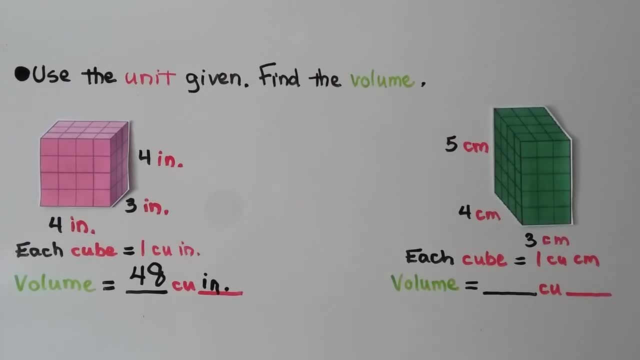 12 times 5. That's 60.. Each cube is 1 cubic centimeter, So the volume is 60 cubic centimeters. The length can be made to fit 1 cube. We have 7 centimeters. We have 7 centimeters. 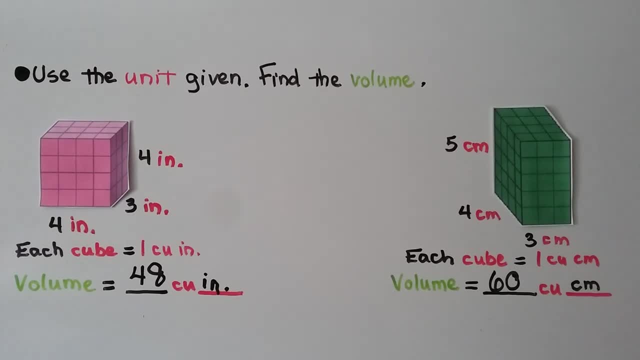 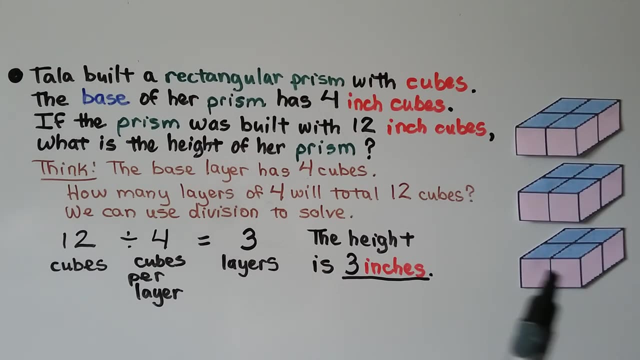 cubes were in the base. we multiplied it by the height. Tala built a rectangular prism with cubes. The base of her prism has four inch cubes. If the prism was built with 12 inch cubes, what's the height of her prism? So we think the base 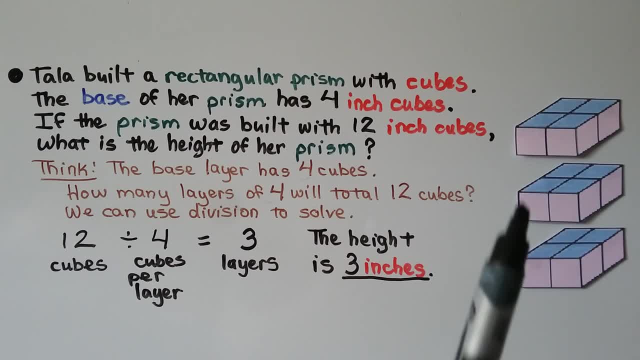 layer has four cubes. How many layers of four will total 12 cubes? We can use division to solve, So this is a very easy problem. You might have one that says the base of the prism has 24 cubes and it'll give you that it has hundreds of cubes. 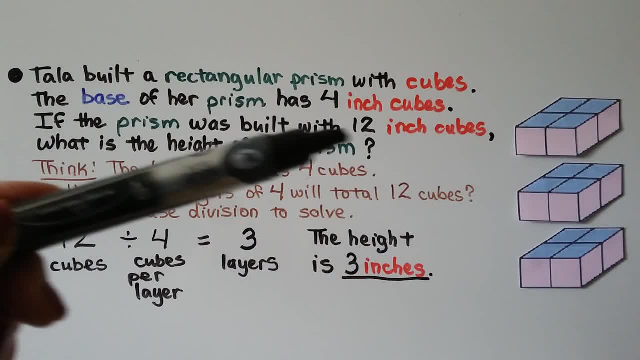 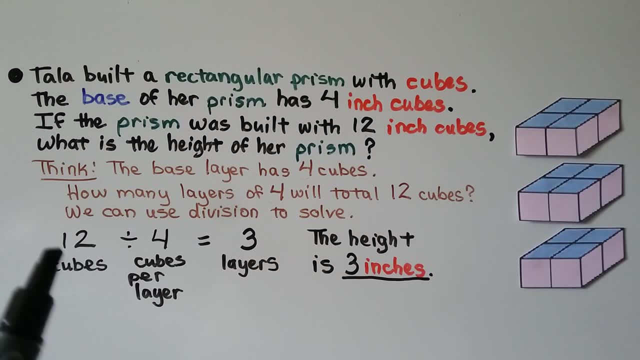 in the entire prism. So I'm using a very easy set of numbers so that you'll understand. We have 12 inch cubes and she has four per layers. That would be three layers And because they're in inches, the height is three inches. If each cube is one inch, the 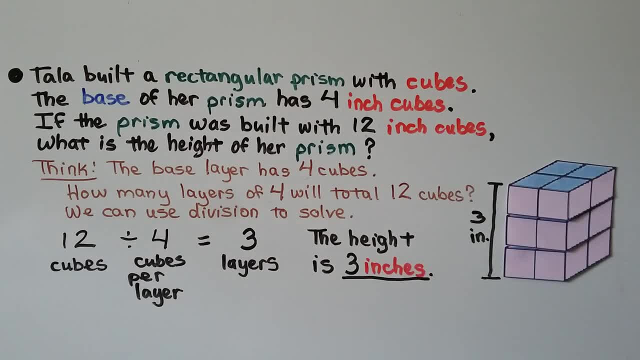 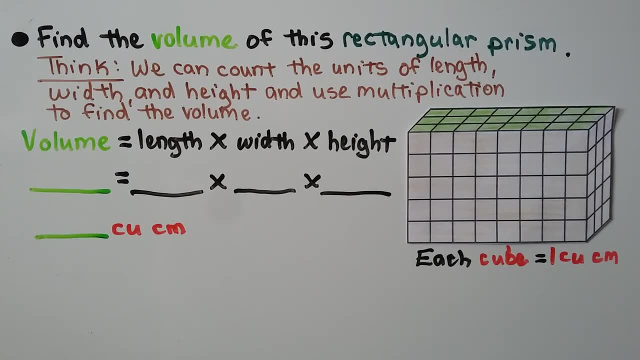 height is one, two, three inches. Find the volume of this rectangular prism. We think we can count the units of length, width and height and use multiplication to find the volume. So it says each cube is 1 cubic centimeter. We count the number. 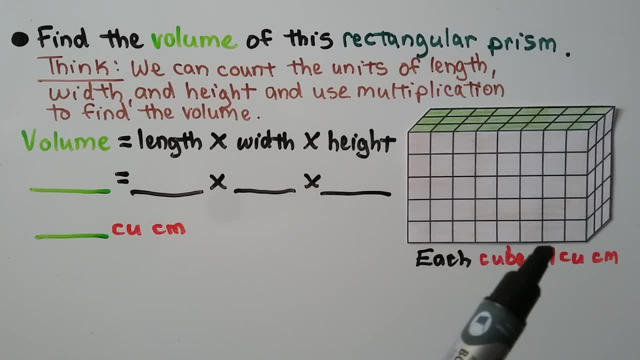 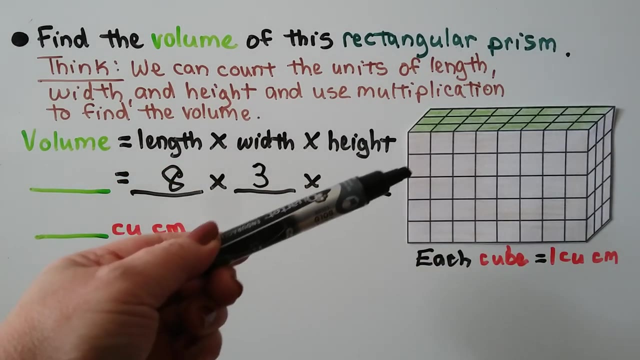 one, two, three, four, five, six, seven, eight. It's got a length of eight. The width is one, two, three. We count the height: One, two, three, four, five. We need to multiply eight.